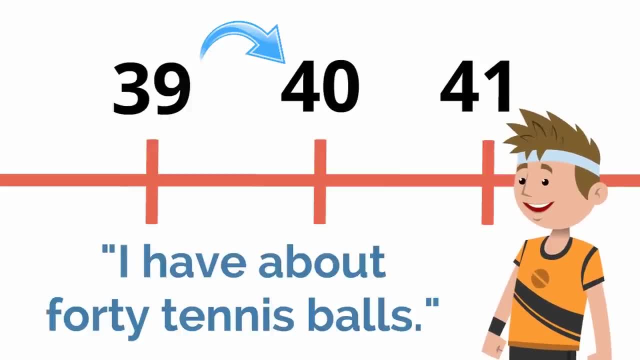 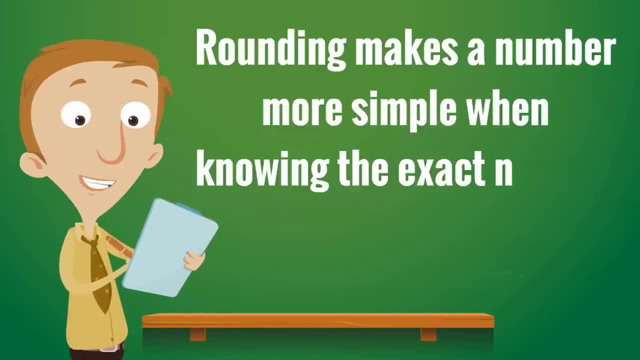 so he answers: I have about 40 tennis balls. That's rounding. Rounding makes a number more simple when knowing the exact number isn't important. That's pretty awesome. Rounding makes a number more simple when knowing the exact number isn't. 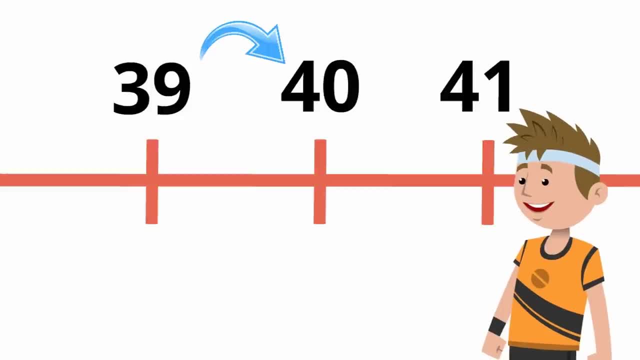 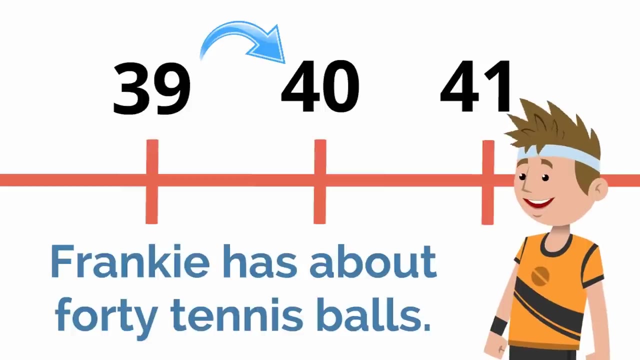 important. In our example, Frankie rounded the number 39 up to the number 40. His friend didn't want to know the exact number of tennis balls. His friend asked for an estimate. Frankie has about 40 tennis balls. Rounding is especially common with bigger numbers, For example. 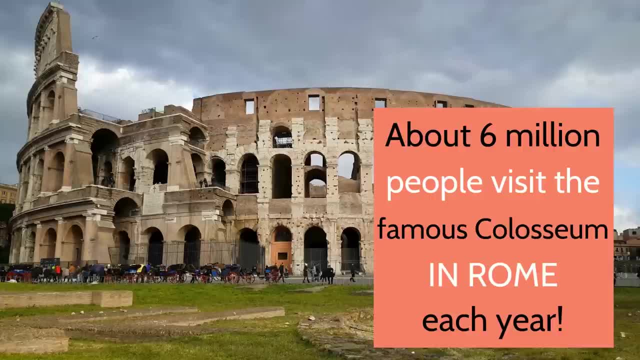 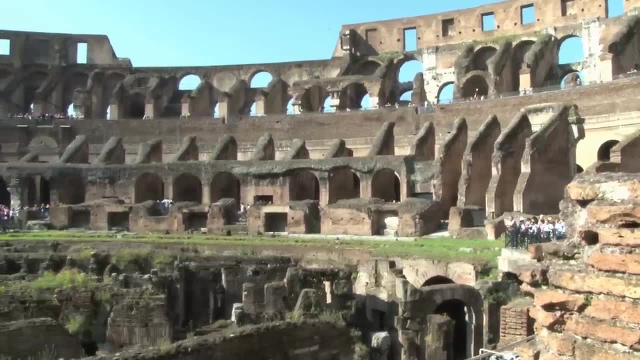 did you know about 6 million people visit the famous Colosseum in Rome each year? Do we know how many people visit the famous Colosseum in Rome each year? Do we know exactly 6 million people visit the Colosseum each year? No, That's why we said about 6 million. 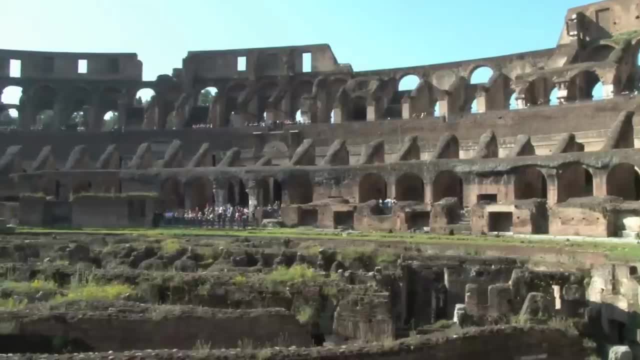 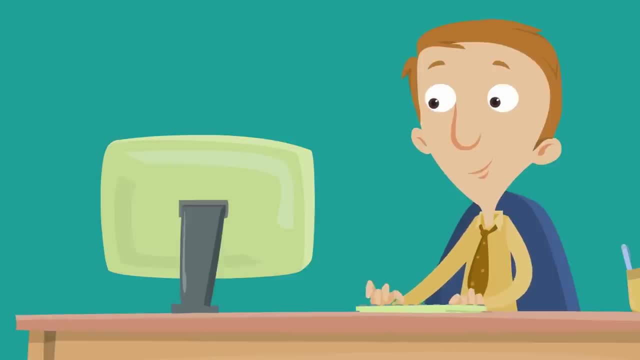 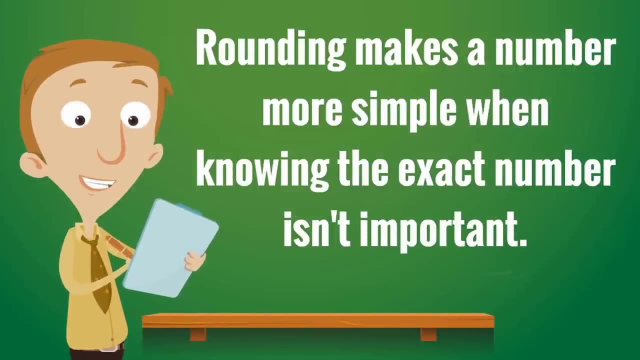 The exact number was rounded so that the number we shared would be simple and easy to remember. That's what rounding does. Rounding makes a number more simple when knowing the exact number isn't important. It's used when we say words like about or roughly We might. 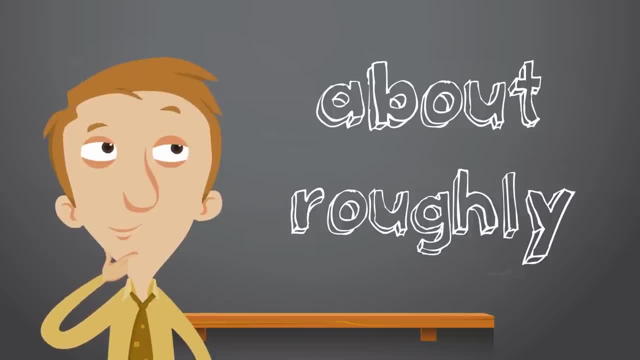 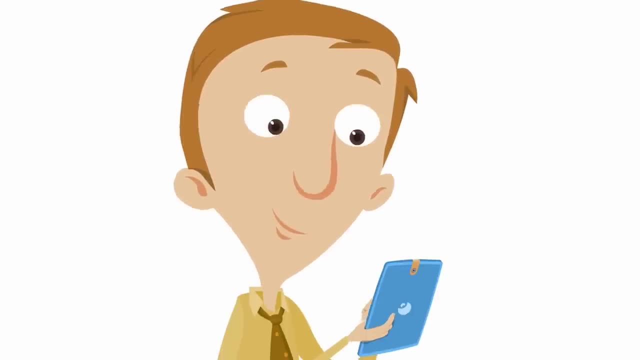 say there are about this many, or there are roughly this many. Okay, now that we know what rounding is and what it does, we need to learn how to round numbers. Let's pick a random number: 46.. Before we do any rounding, we need to review our place values. 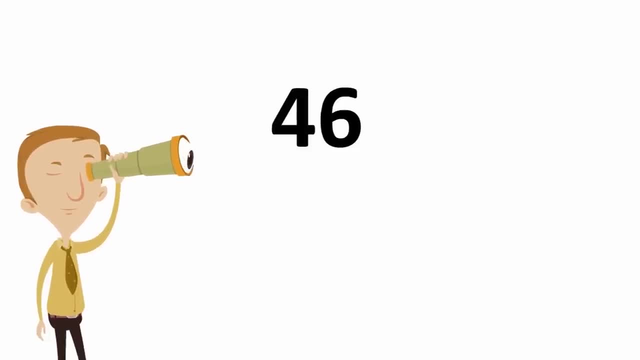 Do you remember place values? It's important to know our place values so we can know exactly how to round. To round the number, What digit is in the ones spot? Yes, the number 6.. This first spot is always the ones spot. What digit is in the tens spot? 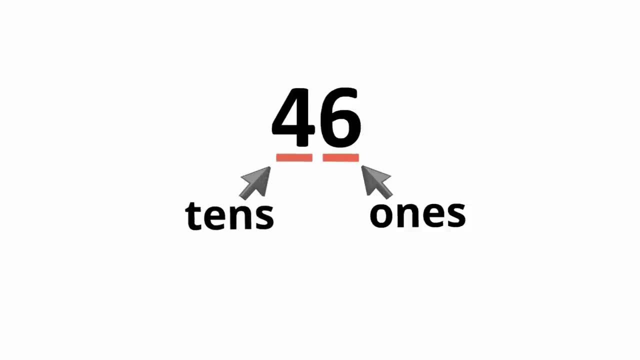 Uh-huh, the number 4.. The second spot is always the tens spot. Great job. Now that we know the place values, let's round 46 to the nearest 10.. You will always have two options: to round up or to round down In this example. 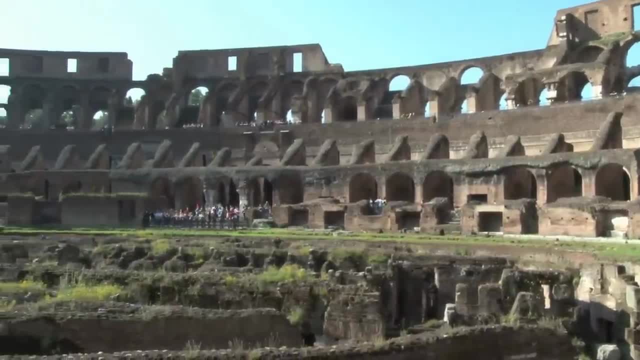 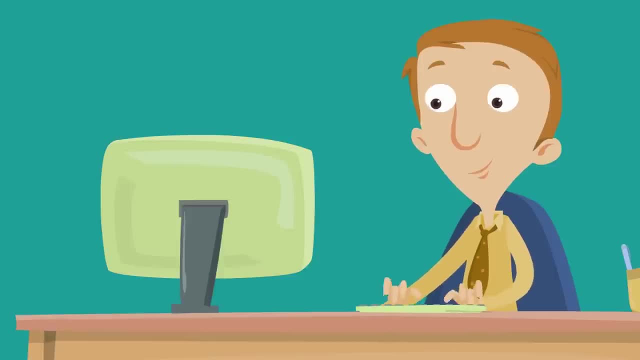 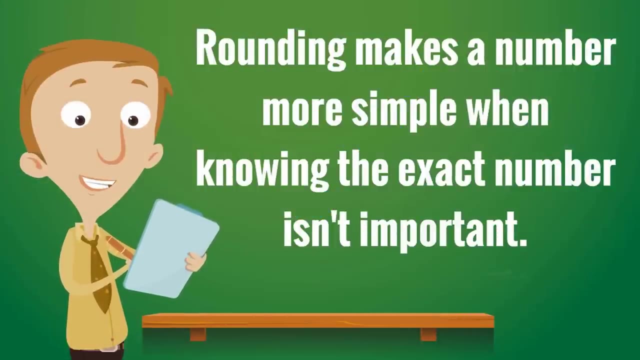 The exact number was rounded so that the number we shared would be simple and easy to remember. That's what rounding does. Rounding makes a number more simple when knowing the exact number isn't important. It's used when we say words like about or roughly. 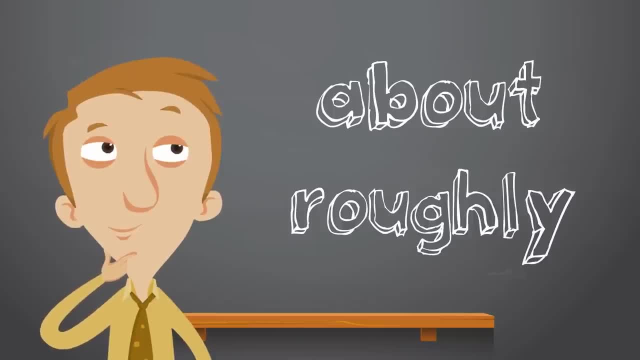 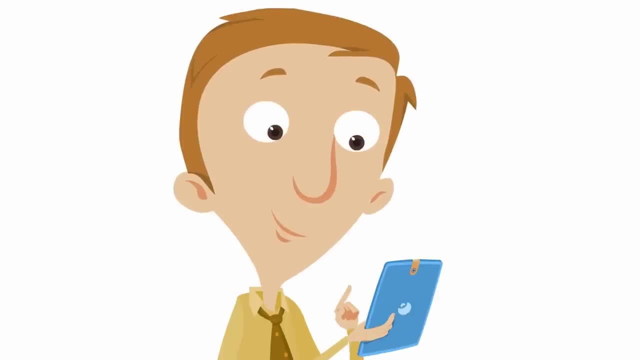 We might say There are about this many, Or There are roughly this many. Okay, now that we know what rounding is and what it does, we need to learn how to round numbers. Let's pick a random number: 46.. 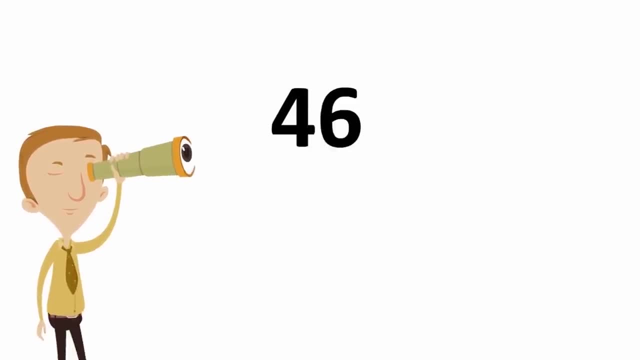 Before we do any rounding, we need to review our place values. Do you remember place values? It's important to know our place values so we can know exactly how to round the number. What digit is in the ones spot? Yes, the number 6.. 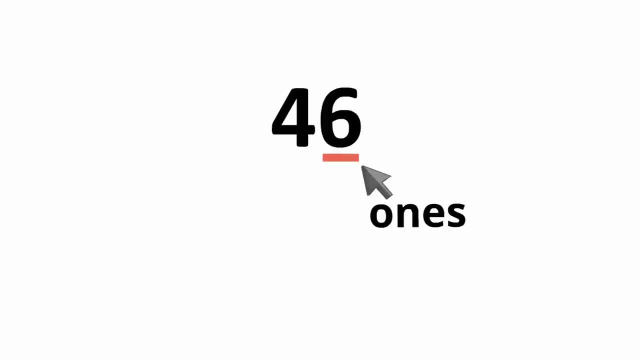 This first spot is always the ones spot. What digit is in the tens spot? Uh-huh, the number 4.. The second spot is always the tens spot. Great job, Now that we know the place values, let's round 46 to the nearest 10.. 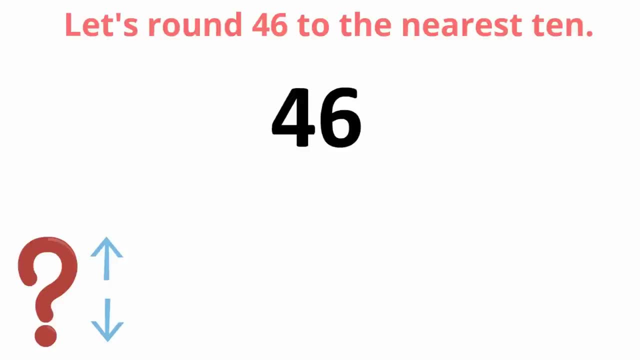 You will always have two options: to round up or to round down. In this example, we will either round up to 50 or we'll round down to 40. But which one do we need to do? To find out, we need to look at the digit before the spot we are rounding to. 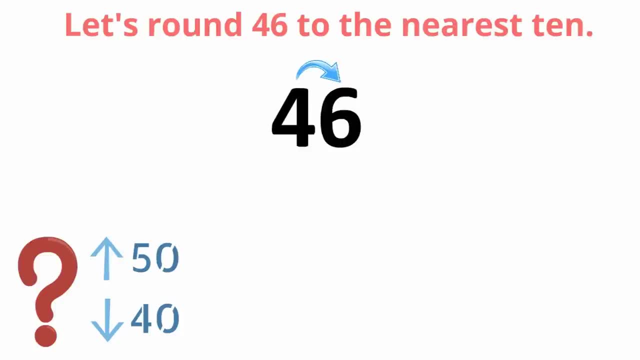 The digit before the 4 is 6.. If you are rounding to the nearest 10, you always look at the ones spot. Okay, here is where we do the trick. If the spot before is 5 or more, round up. 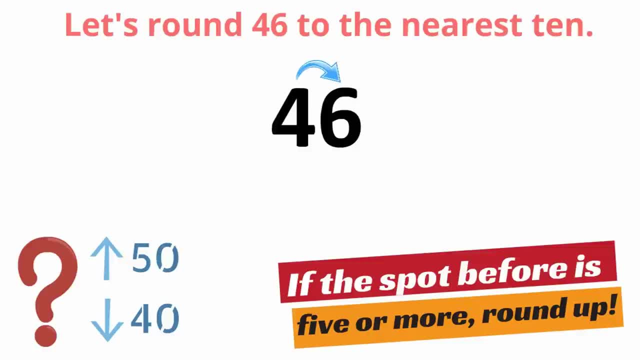 Let's say that again: If the spot before is 5 or more, round up. Alright, so the digit in the ones spot is the number 6.. Are we going to round up or down? Yes, up, So this number will go up to 50.. 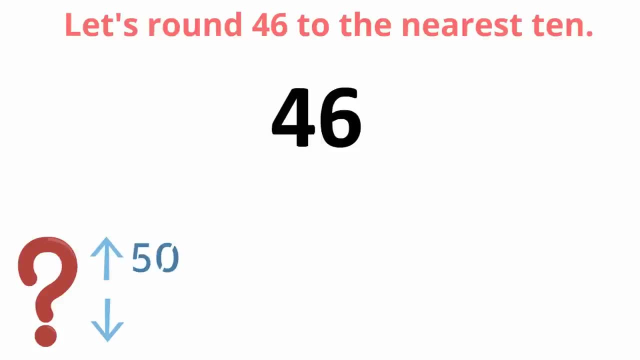 we will either round up to 50 or we'll round down to 40. But which one do we need to do? To find out, we need to look at the digit before the spot we are rounding to. The digit before the 4 is 6.. If you are rounding to the nearest 10, you always look at the one spot. 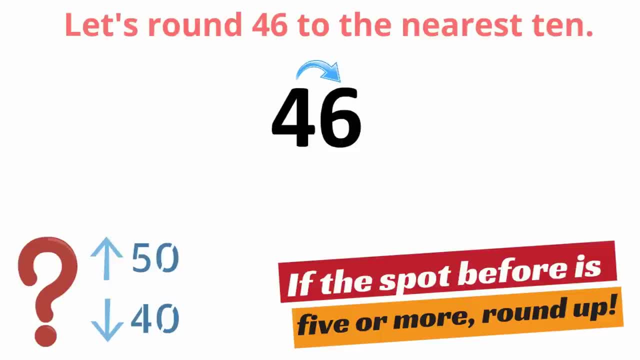 Okay, let's do this. If you are rounding to the nearest 10, you always look at the one spot. Okay, here is where we do the trick. If the spot before is 5 or more round up, Let's say that again: If the spot before is 5 or more round up. 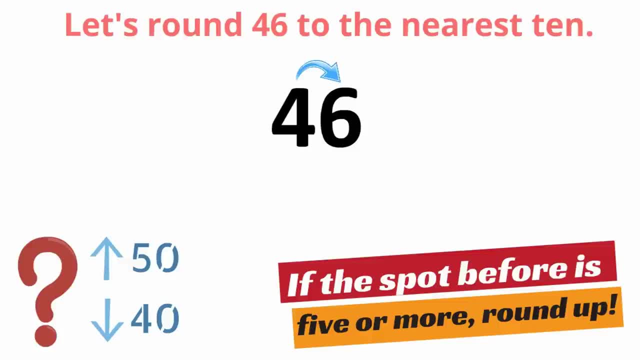 Alright, so the digit in the ones spot is the number 6.. Are we going to round up or down? Yes, up, So this number will go up to 50.. That is the nearest 10.. We did it. We rounded a number 46. 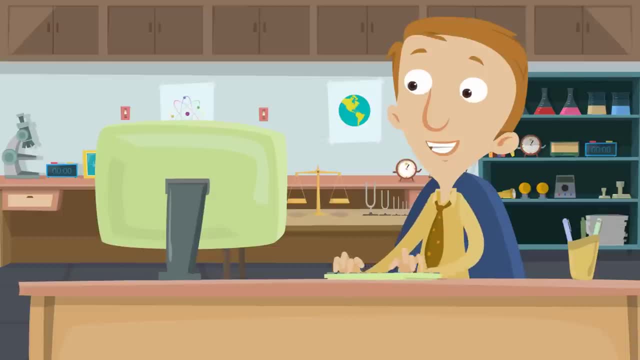 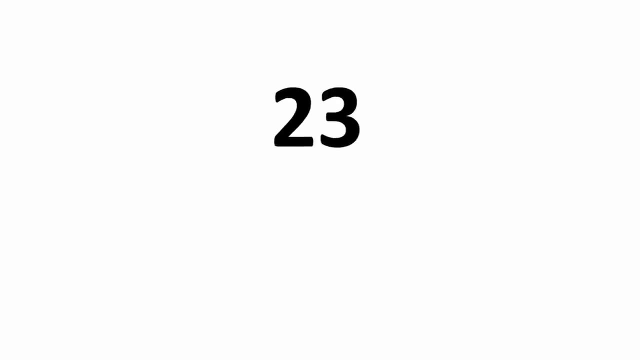 gets rounded up to 50.. You did an awesome job, Let's do another one. Okay, how about the number 23?? What digit is in the one spot? Yes, the number 3.. This first spot is always the one spot. What digit is in the ten spot? 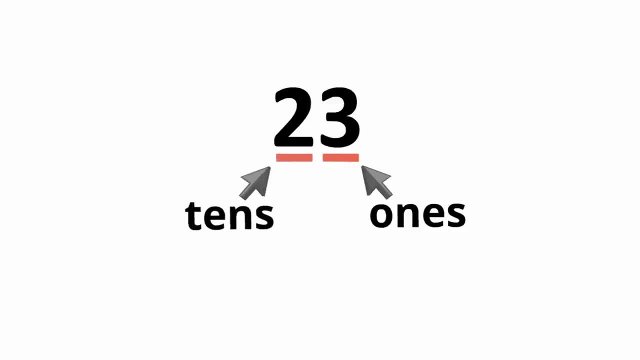 Yes, the number 2,. the second spot is always the ten spot. Now that we know the place values, let's round 21.. How about for the spin for the second spot? Ok, so let's the round again. Are we gonna round up or down? Yes, we are Okay, so this number is always 10.. We rounded up to 50.. That is the nearest 10.. Are we going to round up or down? Let's round up to 50.. That is the number 2, the nearest 10.. Are we going to round up to 500. That is the spot. we are rounding up to the one spot. 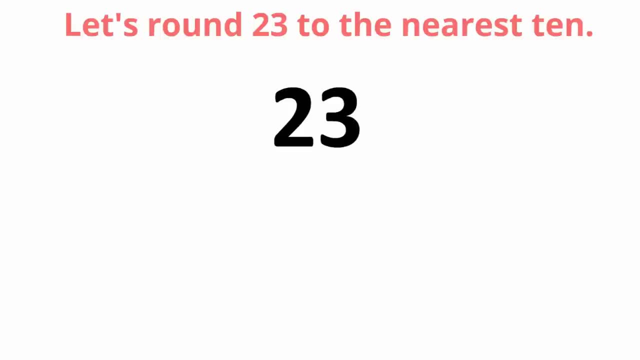 Let's round 23 to the nearest 10.. Remember, you will always have two options: to round up or to round down. In this example, we will either round up to 30 or we'll round down to 20.. Next we need to look at the digit before the spot we are rounding to. 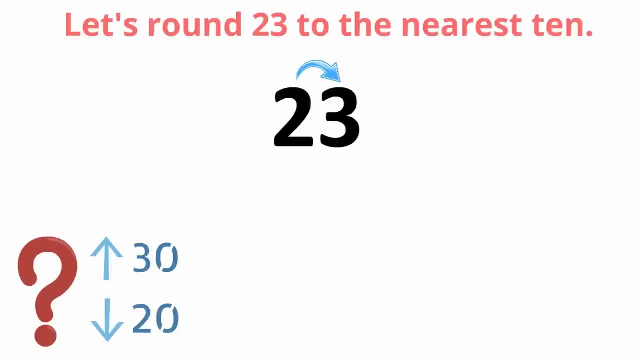 The digit before the 2 is 3.. If you are rounding to the nearest 10, you always look at the 1 spot. Okay, here is where we do the trick. If the spot before is 5 or more round up. That's fun to say. 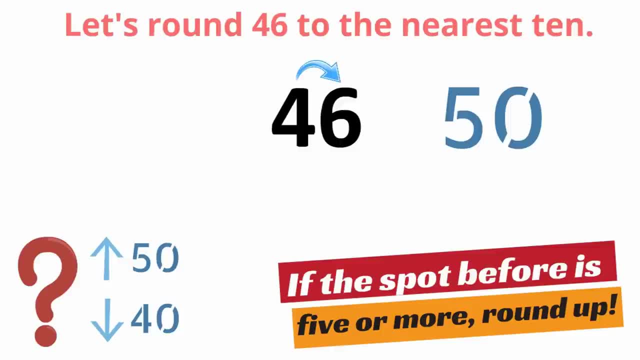 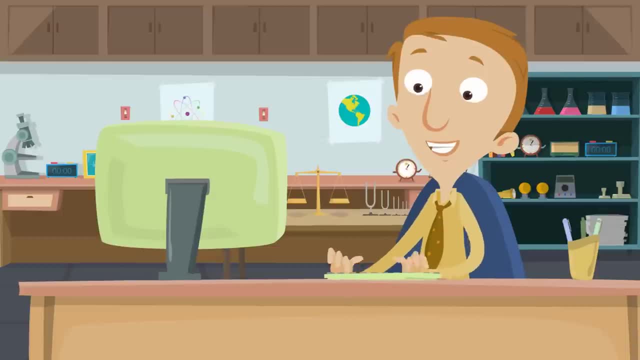 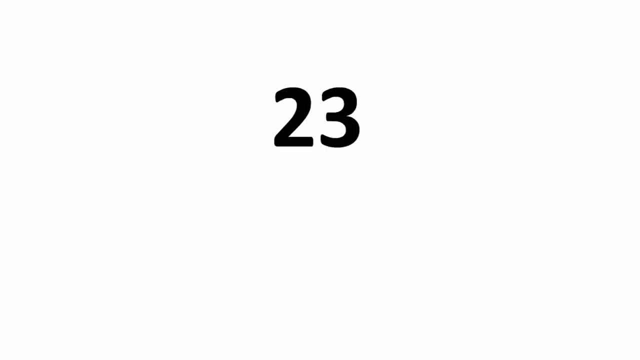 That is the nearest 10.. We did it. We rounded a number. 46 gets rounded up to 50.. You did an awesome job. Let's do another one. Okay, how about the number 23?? What digit is in the ones spot? 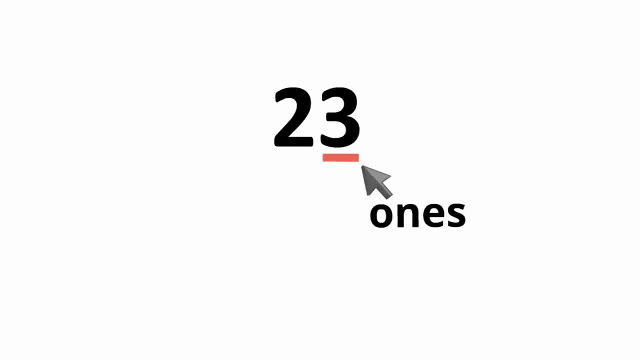 Yes, the number 3.. This first spot is always the ones spot. What digit is in the 10 spot? Yes, the number 2.. The second spot is always the 10 spot. Now that we know the place values, let's round 23 to the nearest 10.. 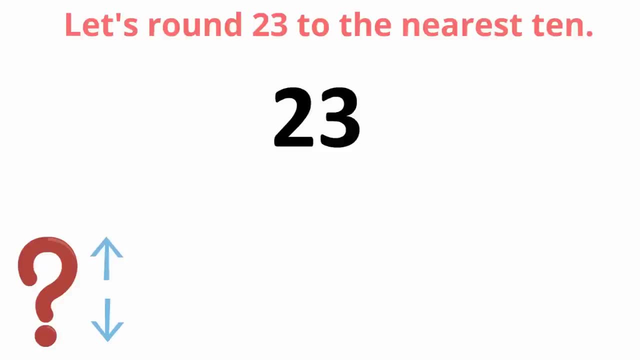 Remember, you will always have two options: to round up or to round down. In this example, we will either round up to 30 or we'll round down to 20.. Next, we need to look at the digit before the spot we are rounding to. 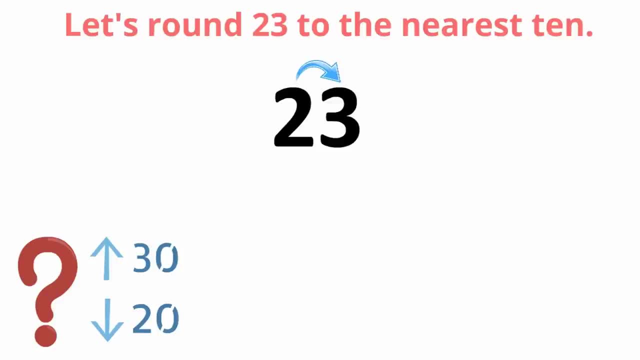 The digit before the 2 is 3.. If you are rounding to the nearest 10, you always look at the ones spot. Okay, here is where we do the trick. If the spot before is 5 or more, round up. 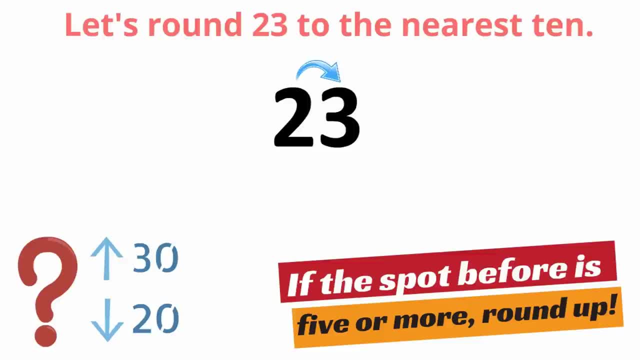 That's fun to say. Let's say it one more time: If the spot before is 5 or more, round up Alright. so the digit in the ones spot is the number 3.. Are we going to round up or down? 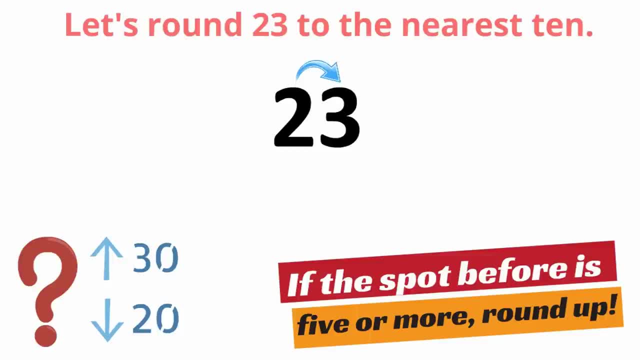 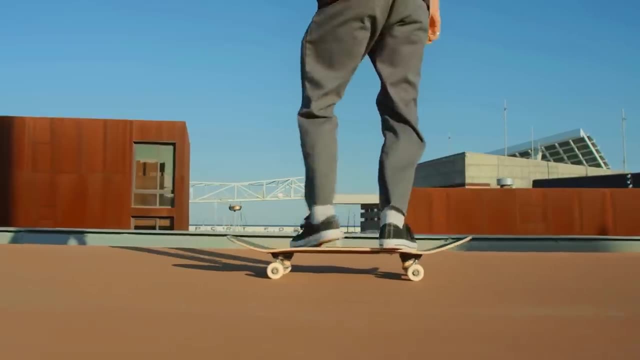 Yes down, So this number will go down to 20.. That is the nearest 10.. That's how you round numbers. 23 gets rounded down to 20.. Great job, Let's use the trick on an even bigger number, because it always works. 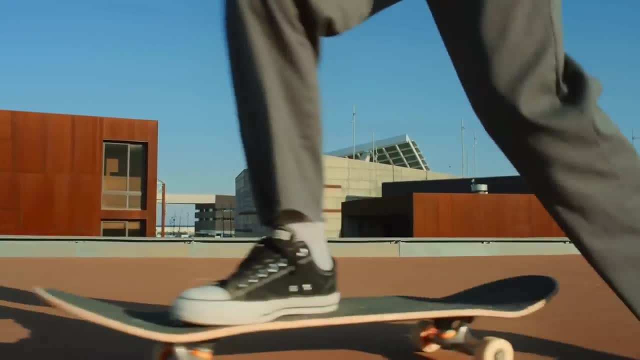 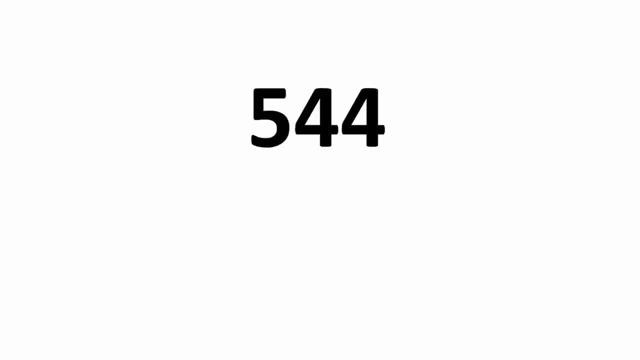 no matter how big the number is. Okay, how about the number 544?? What digit is in the tens spot? Yes, the number 4.. Remember, the second spot is always 4.. The third spot is always the tens spot. 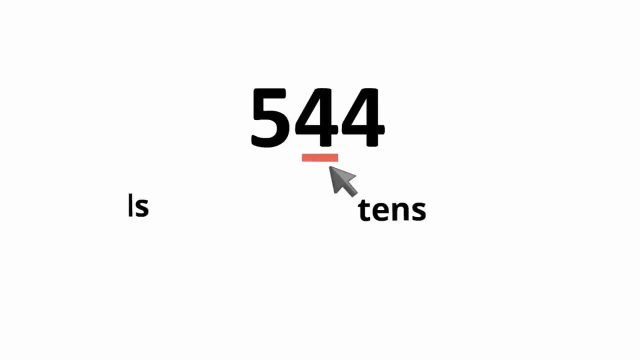 What digit is in the hundreds spot? Yes, the number 5.. The third spot is always the hundreds spot. Now that we know the place values, let's round 544 to the nearest hundred. You will always have two options: To round up or to round down. 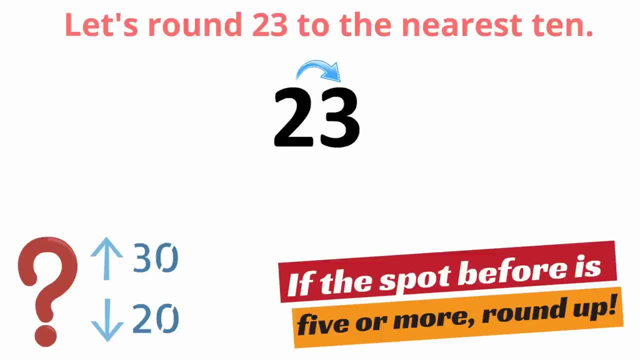 Let's say it one more time: If the spot before is 5 or more, round up. Alright, so the digit in the 1 spot is the number 3.. Are we going to round up or down? Yes, down. So this number will go down to 20.. 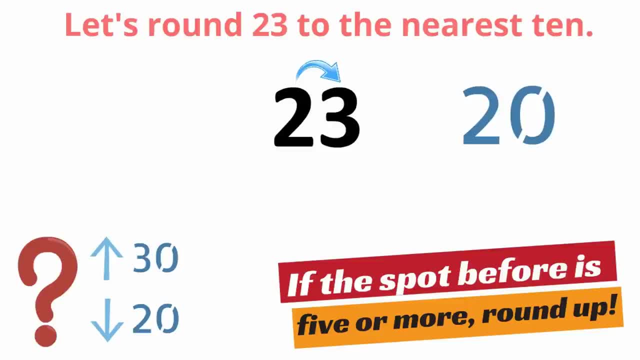 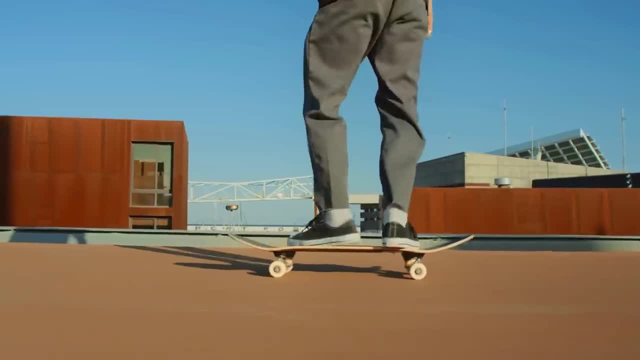 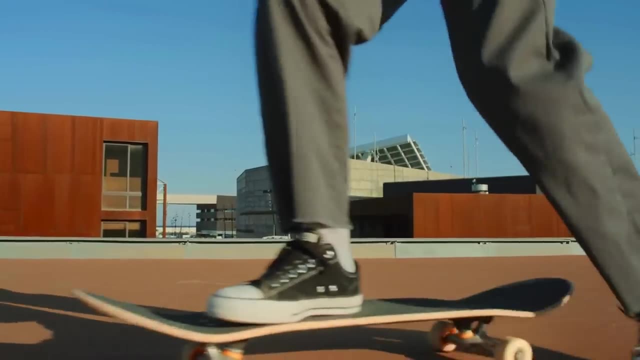 That is the nearest 10.. That's how you round numbers. 23 gets rounded down to 20.. Great job, Let's use the trick on an even bigger number, because it always works, no matter how big the number is. Okay, how about the number 544?? 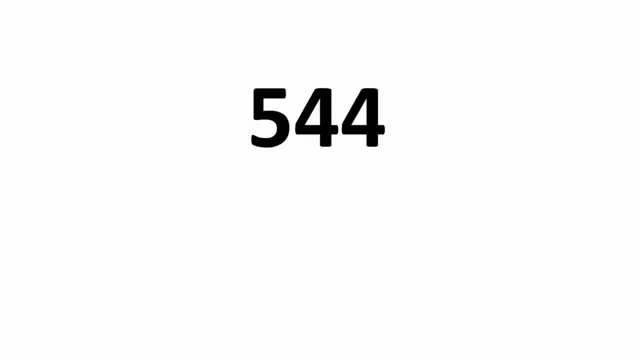 What digit is in the 10's spot? Yes, the number 4.. Remember, the second spot is always the 10's spot. What digit is in the 100's spot? Yes, the number 5.. The third spot is always the 100's spot. 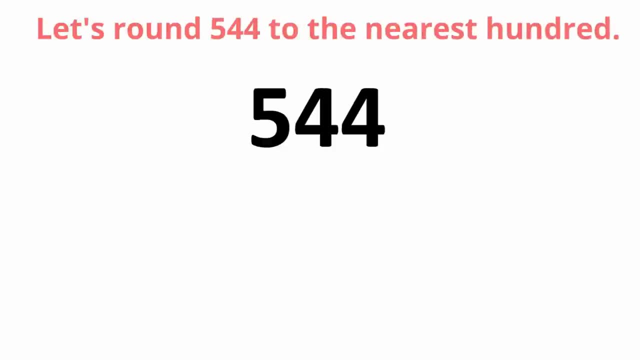 Now that we know the place values, let's round 544 to the nearest 100.. You will always have two options: To round up or to round down. In this example, we will either round up to 600 or we'll round down to 500.. 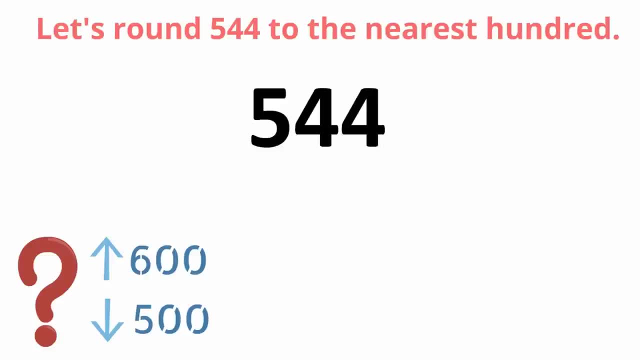 But which one do we need to do? Well, we need to round up. We need to look at the digit before the spot we are rounding to The digit before the 5 is 4.. If you are rounding to the nearest 100, you always look at the 10's spot. 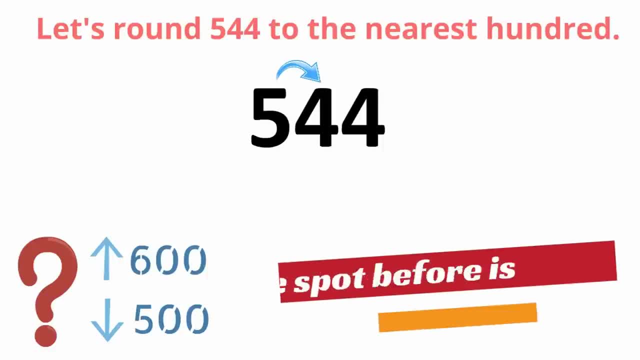 Are you ready for the trick? You know it now. If the spot before is 5 or more round up, That's fun to say. Let's say it again together: If the spot before is 5 or more round up. 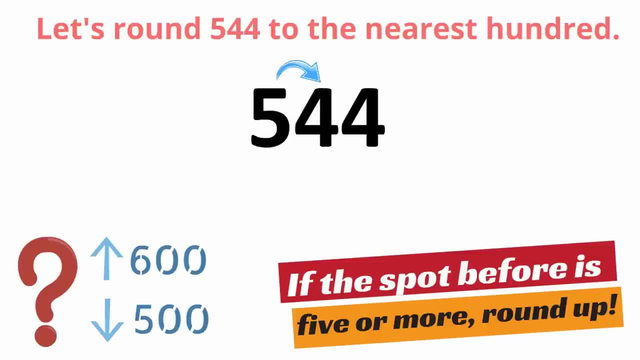 Cool, Okay, So The 10's spot is the number 4.. Are we going to round up or down? Yes, down, So this number will go down to 500.. That is the nearest 100.. And that's how you round numbers. 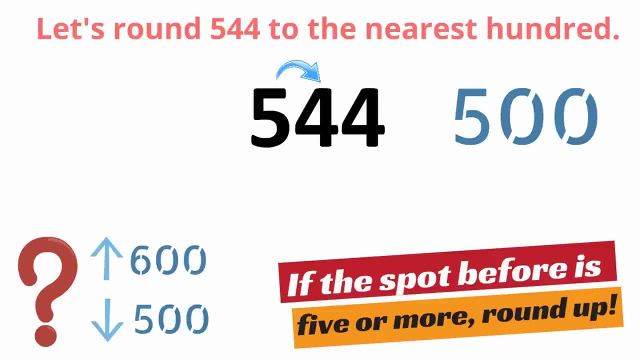 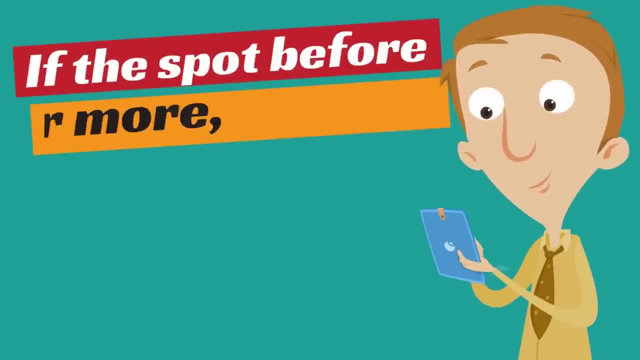 544 gets rounded down to 500.. Now you know the trick to round any number. If the spot before is 5 or more round up. If the spot before is 5 or more round up. Great job You did awesome.